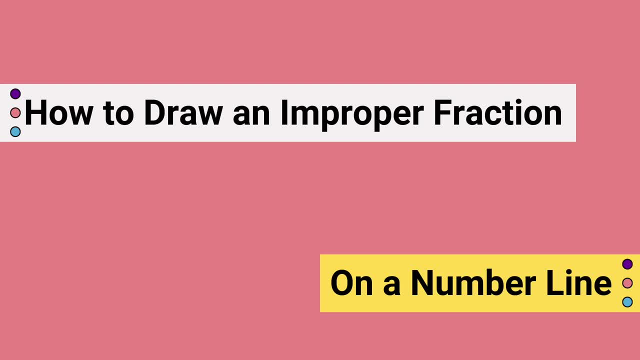 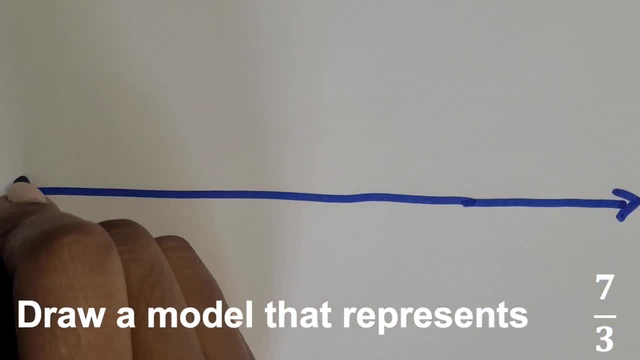 How to draw an improper fraction or a fraction greater than one on a number line. This time we're not using grid paper, We're back to blank paper, or if you have a whiteboard. So we're going to draw our line again and then draw our tick marks. So our first endpoint is zero. Our second 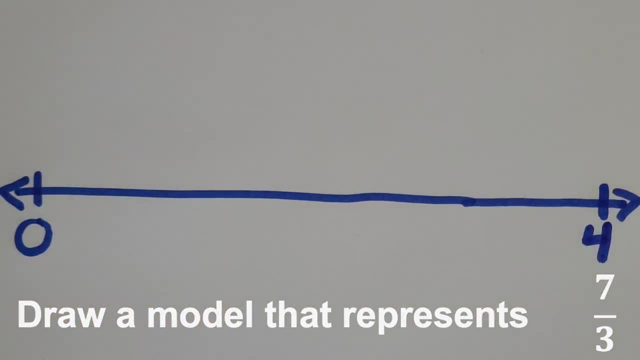 endpoint is four because we need seven thirds. So with our four holes, this time in the middle is going to represent two, and then when you partition each side in half, that first tick mark on the left will be one hole and the tick mark on the right would be three holes. Then we're 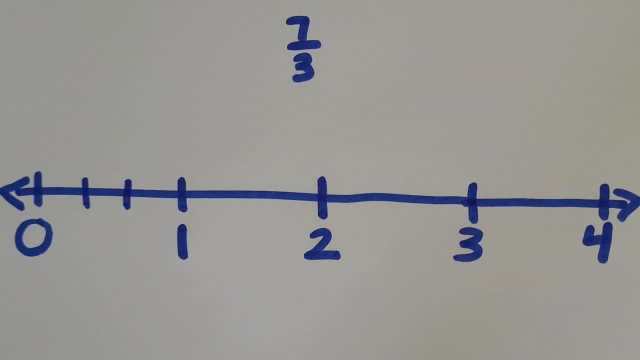 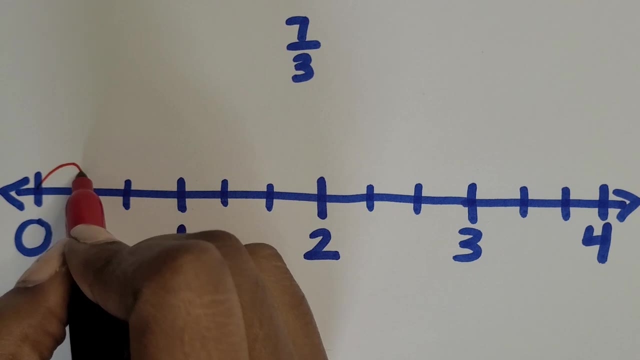 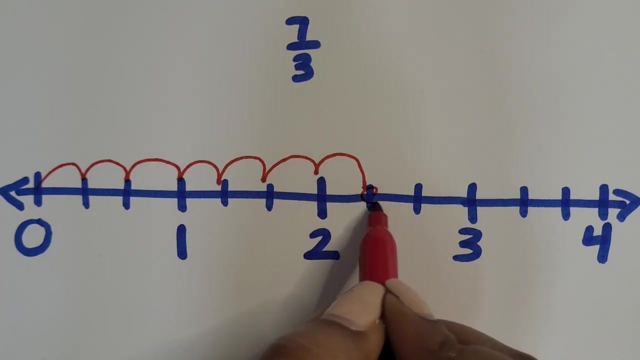 going to partition each hole into thirds and we're going to go from zero all the way to seven thirds. So you can have your students count with you: zero, one third, two thirds, three thirds, which is the same as one hole. four thirds, five thirds, two, which is six thirds, and then seven thirds and then go back and label them. 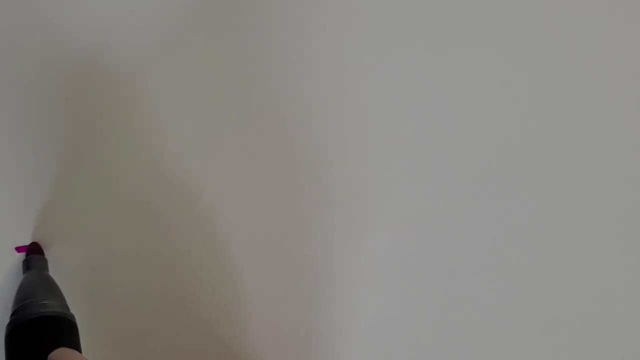 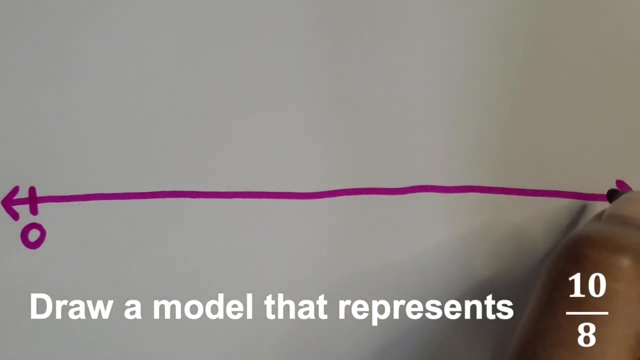 Now we'll represent 10 eighths. So since it's a fraction that's larger than one hole, we know we need at least two holes, So we're going to partition our line into two holes. So zero is the first endpoint, two is the second endpoint, and then in the middle, instead of it being a half. 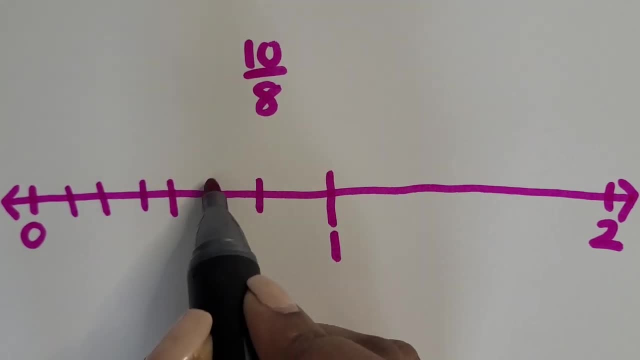 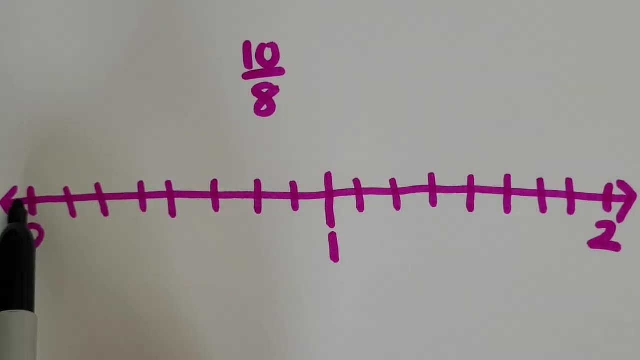 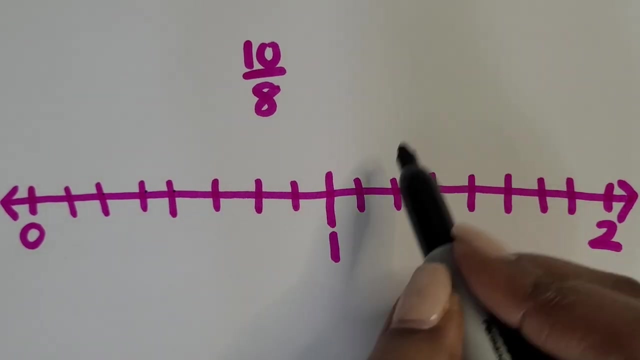 it's going to be one hole, Then we're going to partition each hole, each side, into eighths. You start by partitioning it in half, then into fourths, then into eighths, and then we're just going to count out to 10 eighths and then go back and label them. 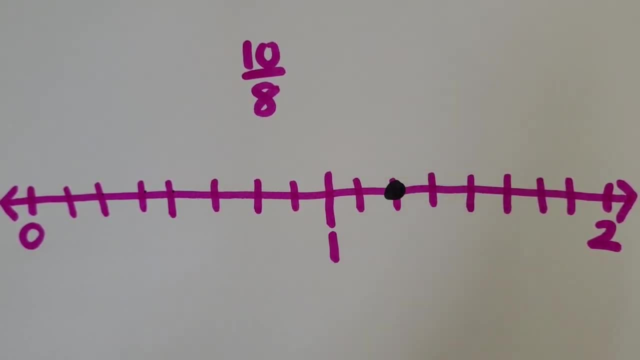 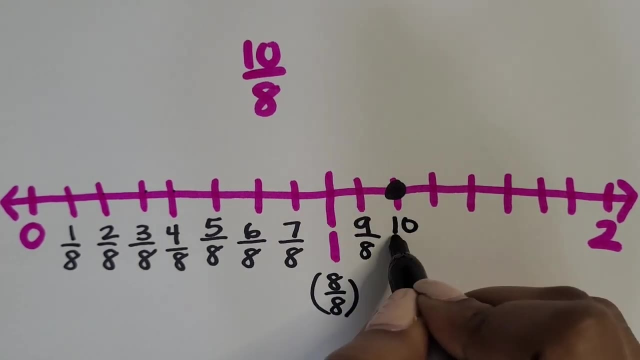 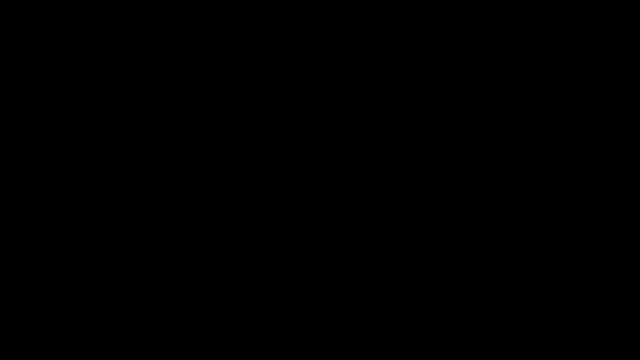 Again, you can label or have your students label the entire number line, all the tick marks or just the point to represent the given fraction. So in the second crack, zero, who are the classes filming this? There's only eight classes, All right. So in the seconddiwię, Let's say, if we were going to treat white셔서 as an Jessie, you know what I've got to do. I've got to be. I've got to be open sheet In a hundred different scales. I'm going to be able do the Biennial. but I'm not going to be able do the German faisio. Yeah, I know I'm going to do a thing.